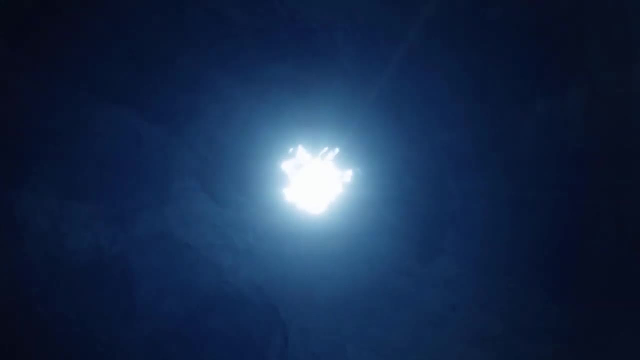 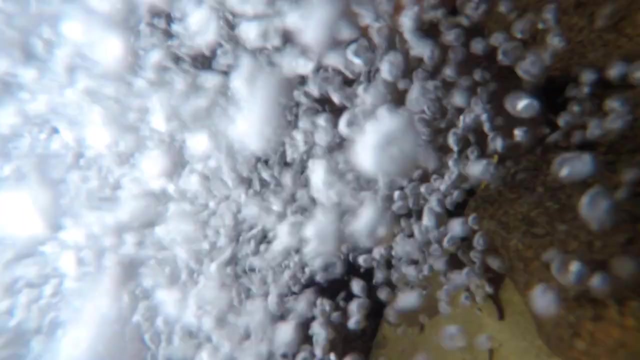 in aquatic ecosystems, converting sunlight and nutrients into organic matter through photosynthesis. They are responsible for generating around 50% of the Earth's oxygen, making them essential for the survival of all life on the planet. Sunlight is essential for the survival of all life on the planet. Sunlight is essential. 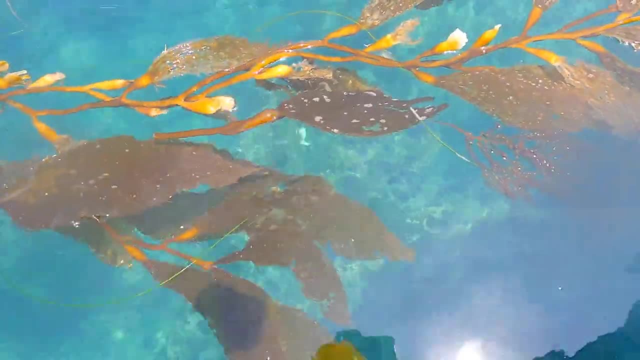 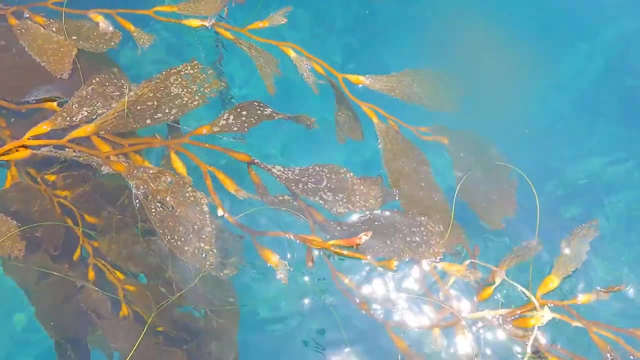 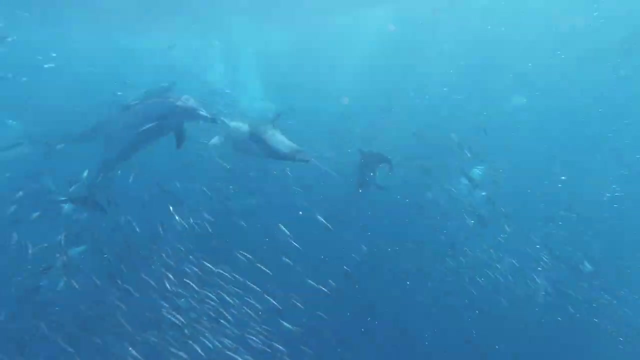 for photosynthesis to occur, Phytoplankton absorbs the energy from sunlight using pigments called chlorophyll, which give them their green color. The oxygen produced by phytoplankton is not just important for humans, it's also essential for marine life. In fact, whales, dolphins, 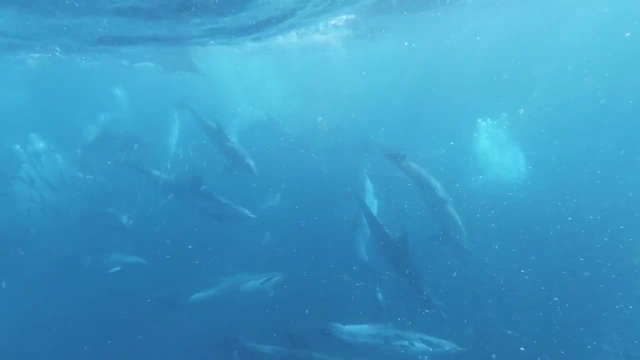 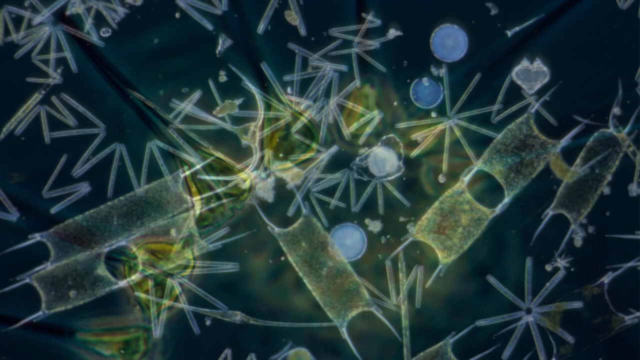 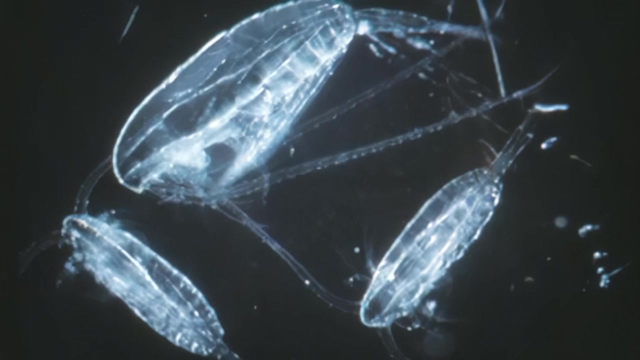 and other marine mammals rely on oxygen produced by phytoplankton for their survival. Despite their small size, phytoplankton are incredibly diverse, with thousands of different species found in oceans around the world. Some species are adapted to survive in the freezing waters of the Arctic, while others thrive in warm tropical waters. 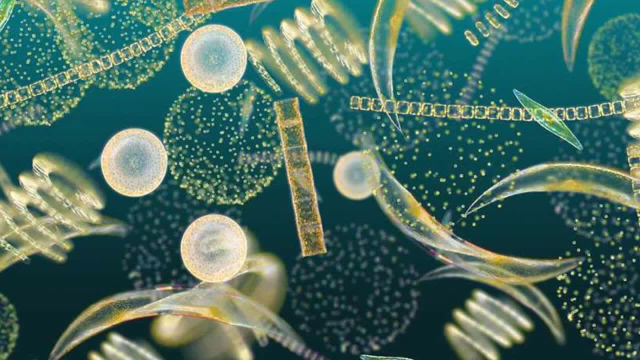 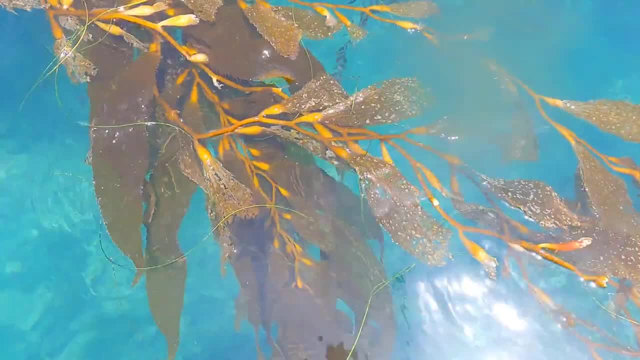 They come in a variety of shapes, from tiny spheres to long filamentous strands. Phytoplankton is the foundation of the aquatic food chain, providing food from everything from tiny zooplankton to massive whales. Whales feed on krill. 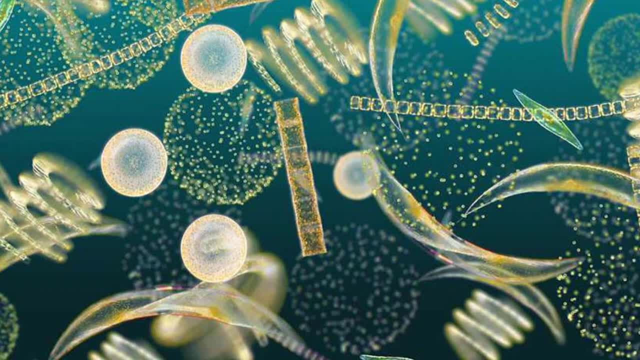 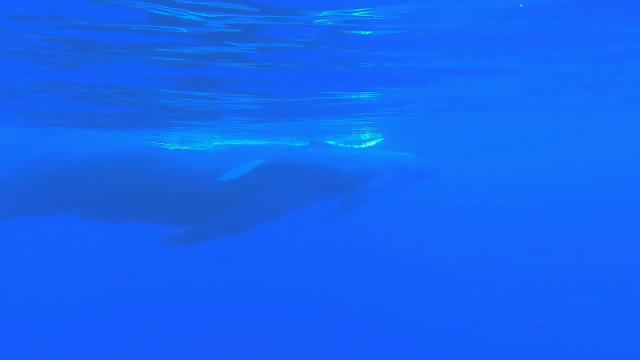 which, in turn, feed on the sea and whales feed on the sea. Phytoplankton are the most important species of the world. Without phytoplankton, krill populations would decline, leading to a chain reaction that would ultimately impact the entire marine ecosystem. 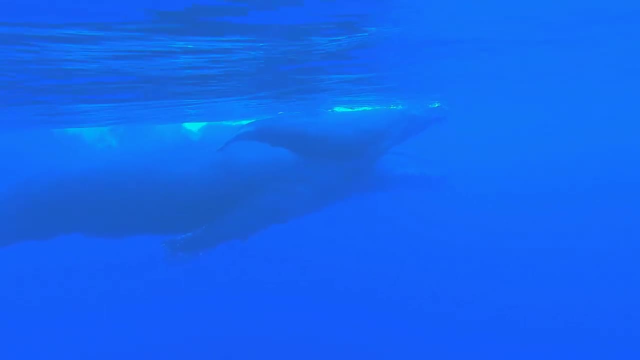 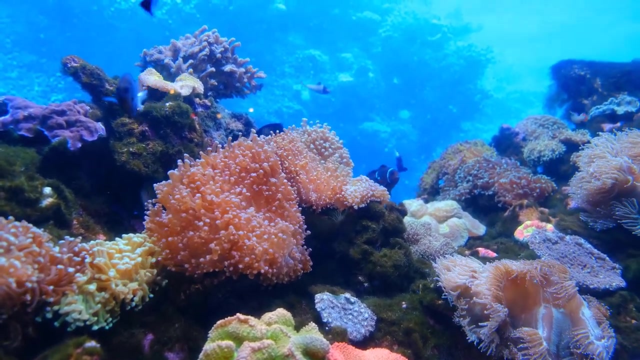 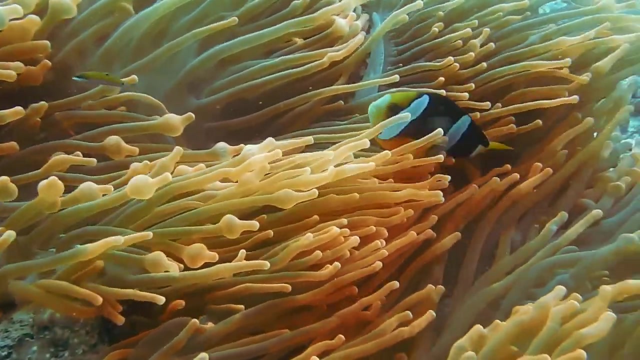 and cause devastating consequences for all life on the planet. It also plays a critical role in maintaining healthy coral reefs. Coral reefs are home to thousands of species of fish and they protect coastlines from storms and erosion, But coral reefs are sensitive to changes in ocean chemistry. such as an increased acidity caused by the absorption of carbon dioxide from the atmosphere. Phytoplankton helps to regulate the ocean's acidity by absorbing carbon dioxide and producing oxygen. But phytoplankton doesn't just provide food for other organisms. They also play a critical role in regulating the Earth's climate Through photosynthesis phytoplankton. 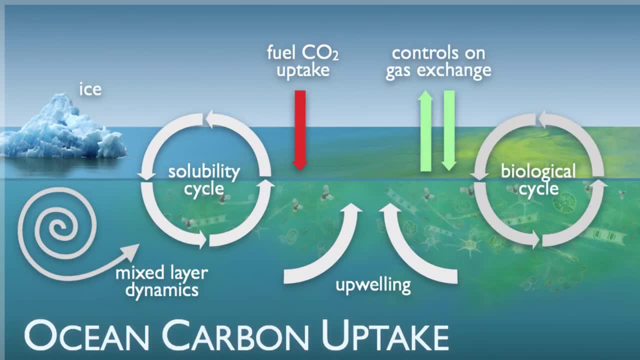 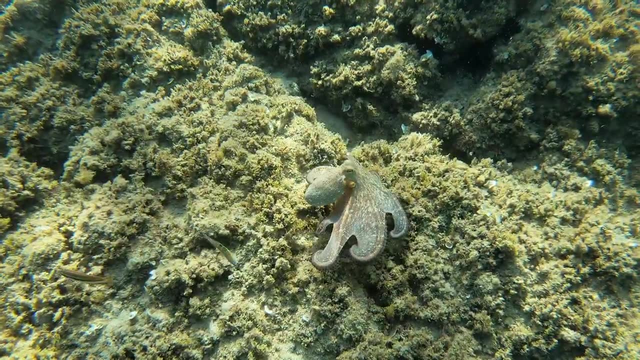 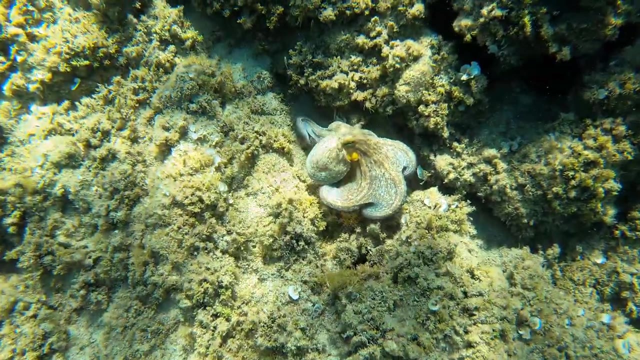 absorbs large amounts of carbon dioxide from the atmosphere, helping to reduce greenhouse gas levels and combat climate change. In addition, phytoplankton are important indicators of environmental health Because they are so sensitive to changes in water temperature, nutrient levels and other environmental factors. changes in the phytoplankton population can 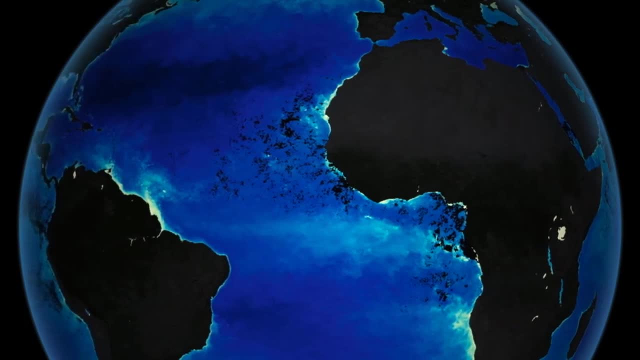 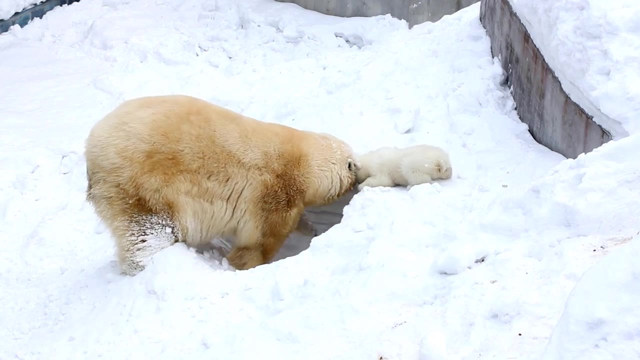 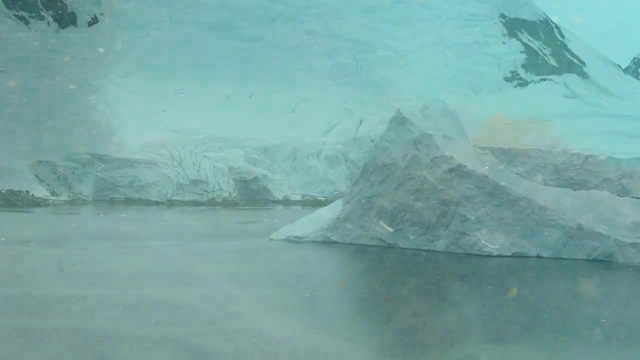 provide early warning signs of larger ecosystem changes. It even has an impact on terrestrial animals like polar bears. Polar bears rely on sea ice for hunting and breeding, But the sea ice melt due to climate change is threatening their survival. Phytoplankton can help to reduce. 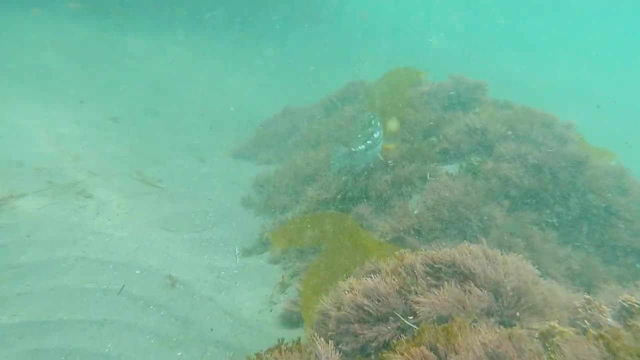 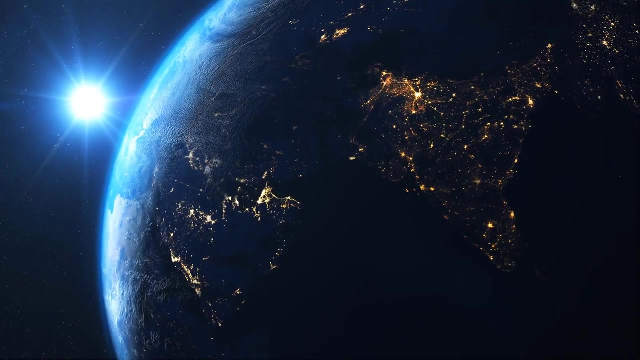 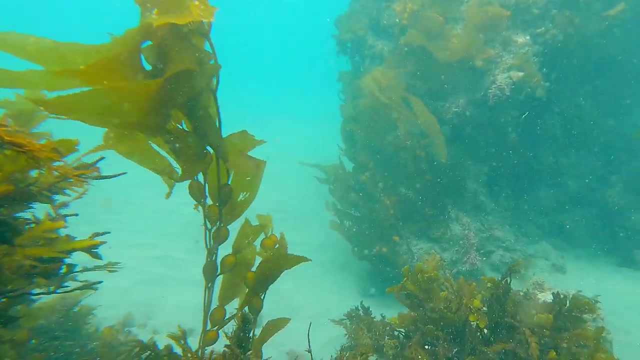 the amount of carbon dioxide in the atmosphere and slow the rate of climate change, which, in turn, can help to protect polar bear populations. Despite their critical importance to the planet, phytoplankton populations are under threat from a range of factors, including climate change, pollution and overfishing, As ocean temperatures continue to. 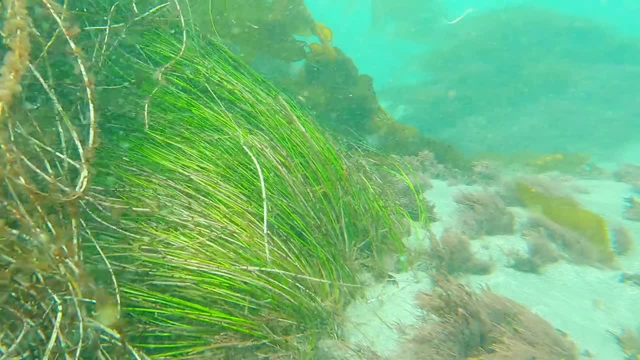 rise. many species are dying for a change in the environment and the range of Iowa's seabirds. many species of phytoplankton are struggling to adapt to changing conditions. Some species are moving toward the poles in search of cooler waters. while others are simply dying off. This is leading to significant changes in the composition of phytoplankton populations, with potential ripple effects throughout the entire ecosystem. Pollution is also a major threat to phytoplankton, as runoff from agricultural and industrial activities can introduce harmful chemicals into the water. This can lead to toxic blooms of algae. 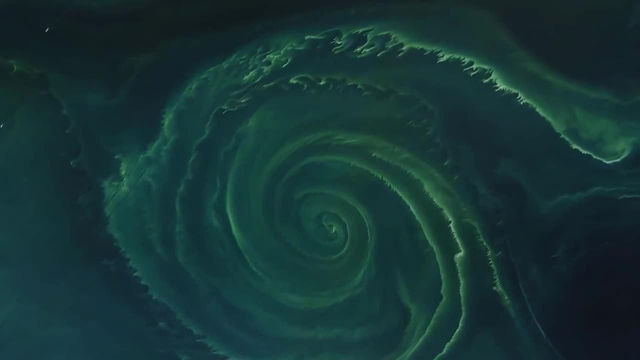 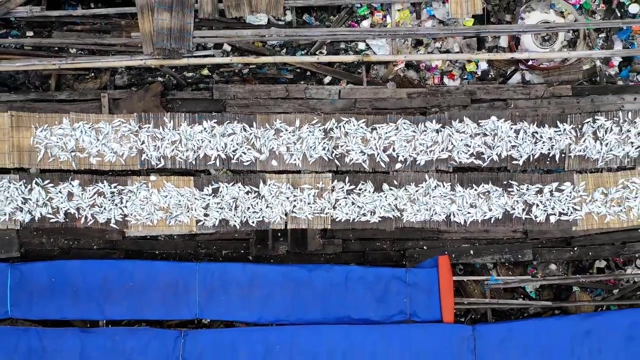 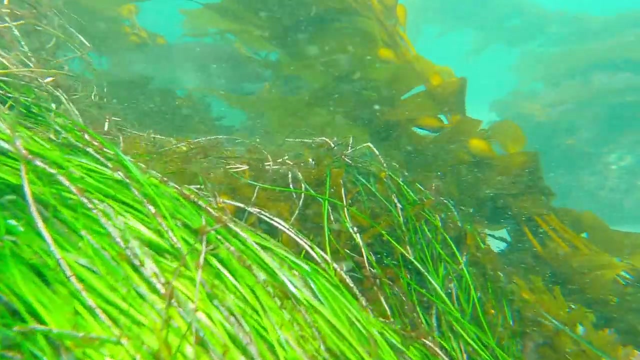 that cause mass die-offs of other marine organisms. Overfishing is another concern, as large-scale removal of fish from the ecosystem can disrupt the delicate balance between predator and prey. This can have knock-on effects on phytoplankton populations, as certain types of 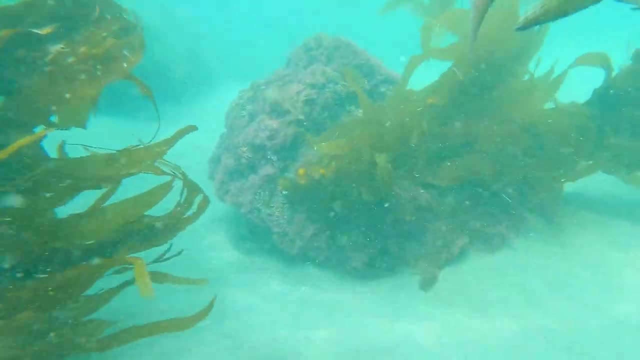 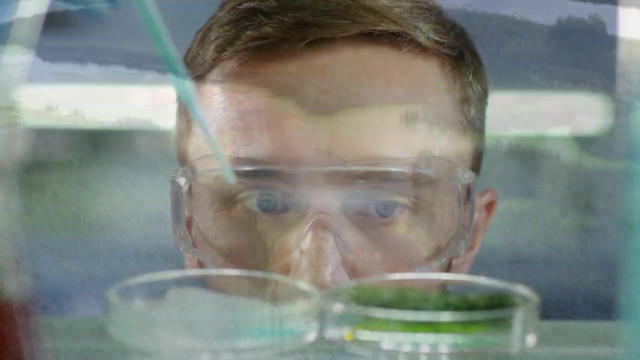 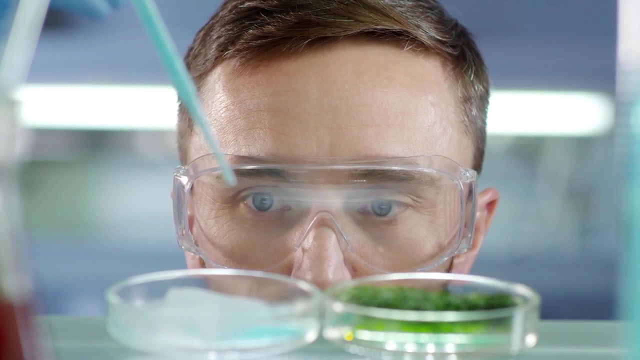 fish are important grazers that help to control the growth of phytoplankton. Despite these threats, there is still hope for the future of phytoplankton. Scientists and conservationists are working to better understand these critical organisms and develop strategies to protect them. But what if we could harness the power of phytoplankton? 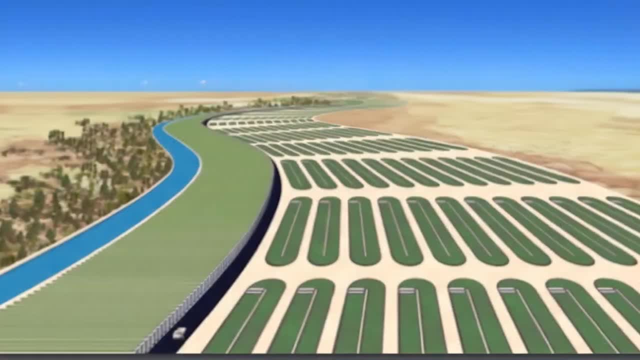 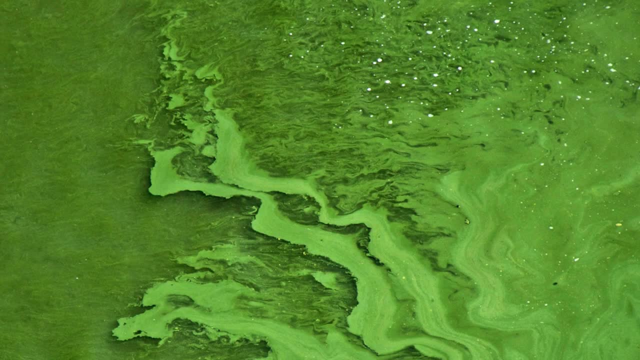 to fight climate change. Scientists are exploring the use of bioenergy from phytoplankton as a renewable energy source. Phytoplankton can be grown in large quantities and harvested for production in the future. Phytoplankton can be grown in large quantities and harvested for 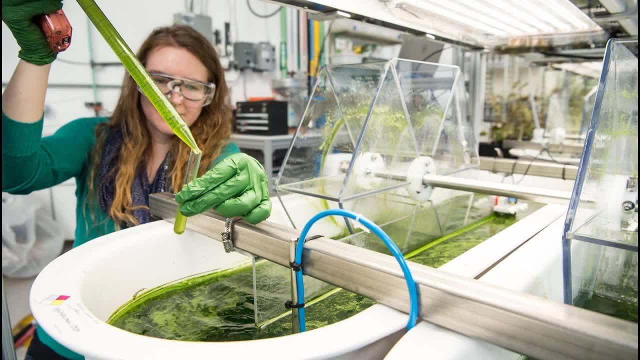 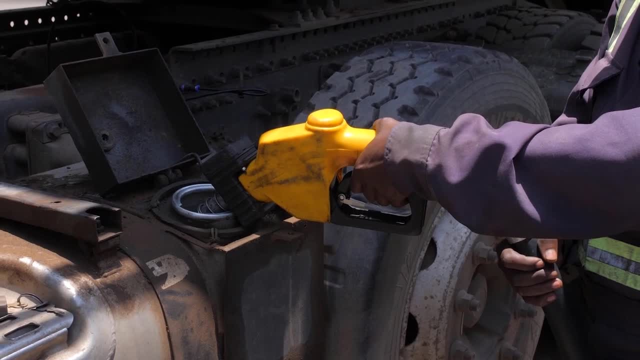 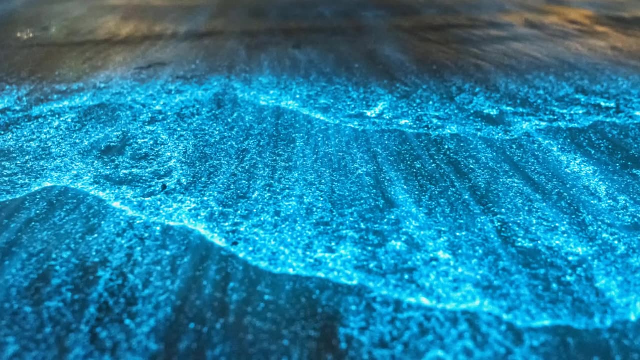 their biomass, which can be converted into biofuels or used to generate electricity. This could help to reduce our dependence on fossil fuels and mitigate the impacts of climate change. Some species are even bioluminescent, meaning they produce their own light. 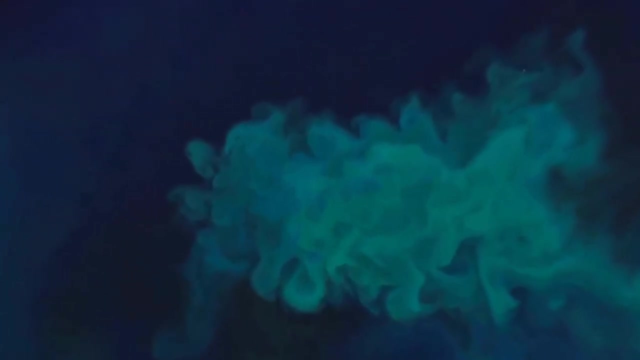 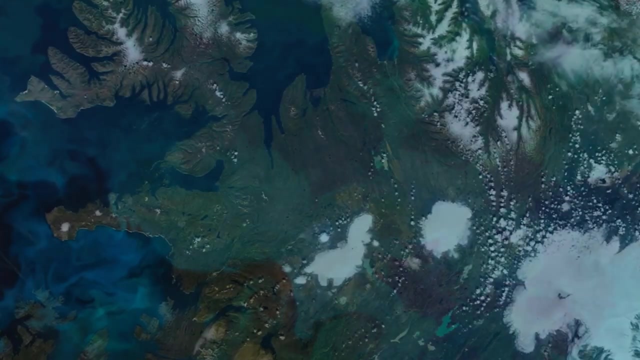 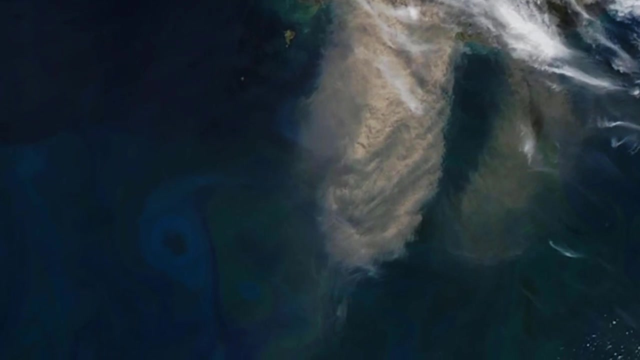 creating a beautiful display in the ocean at night. Another interesting fact about phytoplankton is that they can form massive blooms which can be seen from space. These blooms occur when conditions are just right, with plenty of sunlight and nutrients available. While these 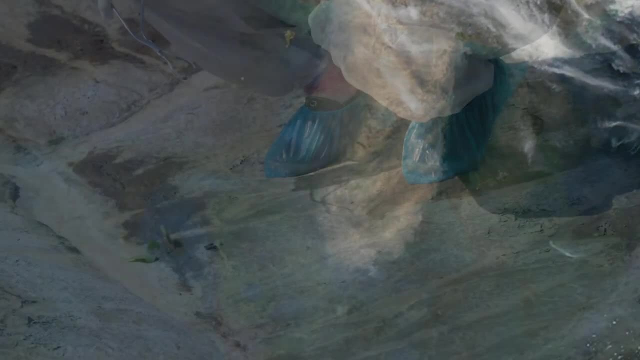 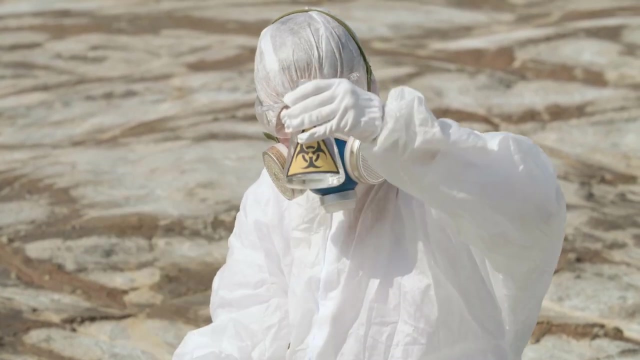 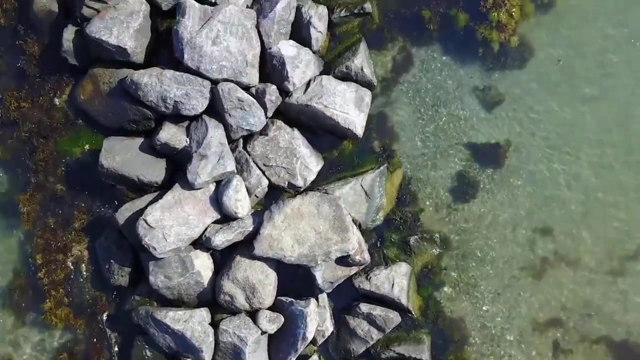 blooms can be beautiful to look at, they can also have negative impacts on the environment. Some phytoplankton species can produce harmful toxins which can be harmful to marine life and even humans if they consume contaminated seafood. Despite these risks, phytoplankton are essential. 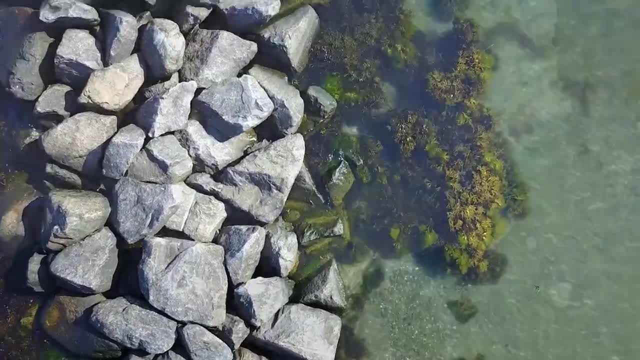 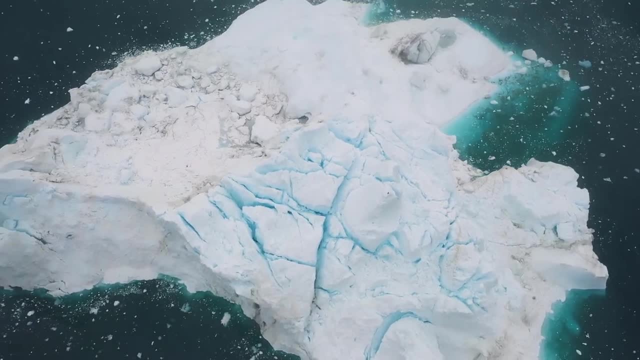 to the health of the ocean and the planet as a whole. As we continue to face the challenges of climate change and environmental degradation, it's more important than ever to understand and appreciate the critical role that these tiny organisms play in keeping our planet alive. 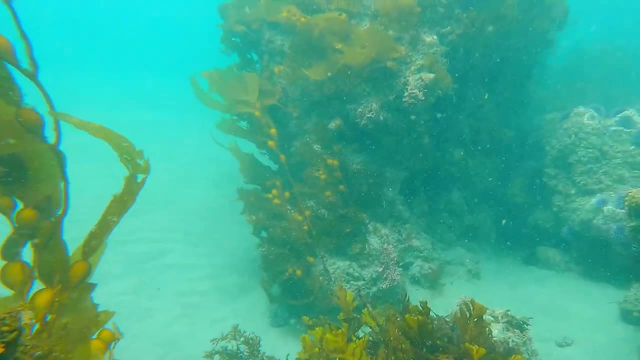 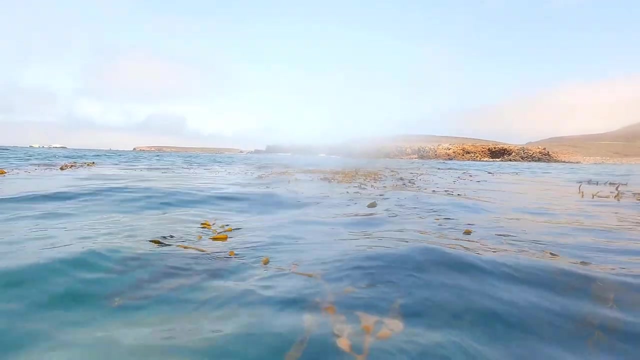 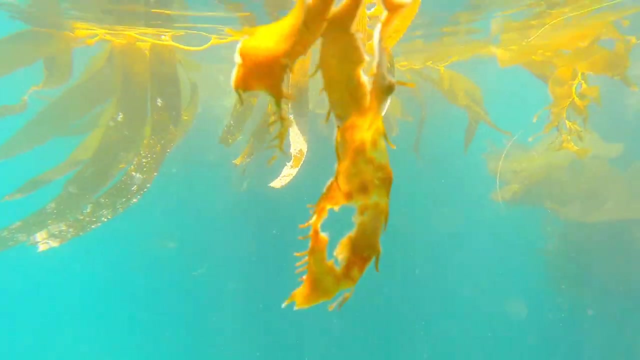 While phytoplankton is the primary source of oxygen in the ocean, other organisms also contribute to oxygen production, like seaweed, which is photosynthetic and produces oxygen through photosynthesis. Algae are another type of photosynthetic organism that can produce oxygen. 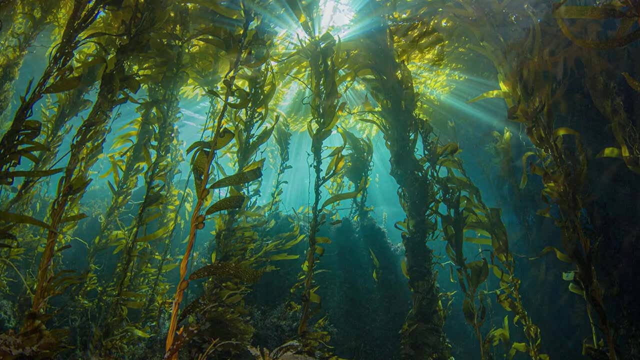 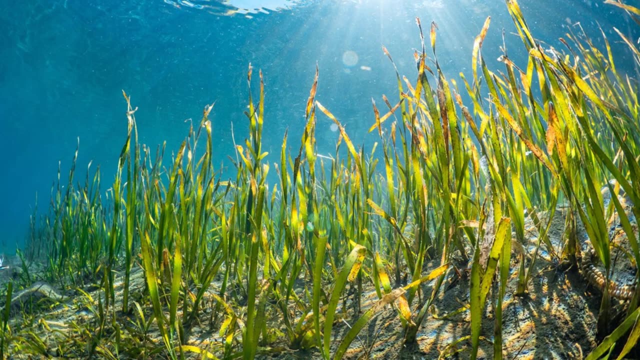 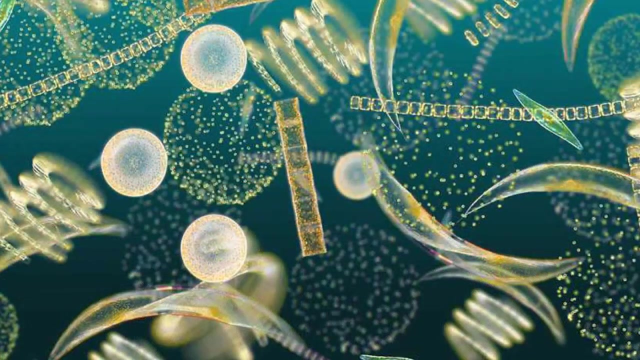 some species of algae, such as kelp, are also important habitats for marine life. Seagrasses are flowering plants that grow in shallow waters. Like other plants, they produce oxygen through photosynthesis. Overall, while phytoplankton is the primary producer of oxygen in the ocean. 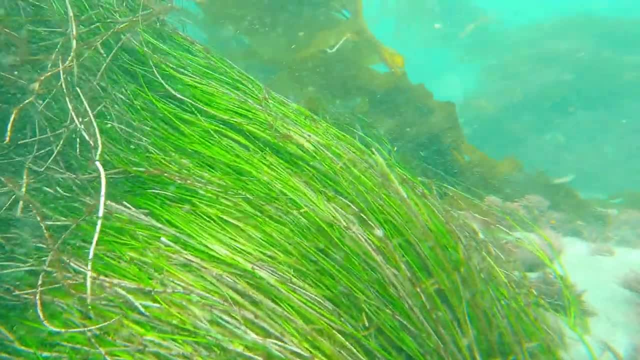 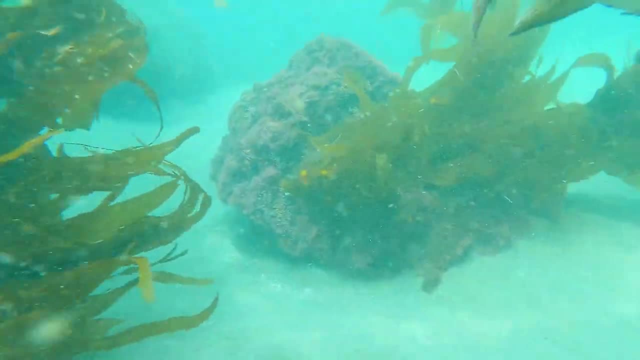 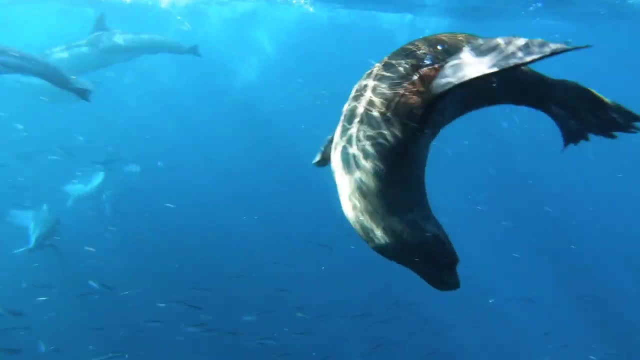 there are a variety of other organisms that contribute to oxygen production and are essential to the health of the ocean ecosystem. In conclusion, phytoplankton may be tiny, but their role in the planet's ecosystem is massive. These microscopic organisms are responsible for producing more than half of the oxygen we breathe. 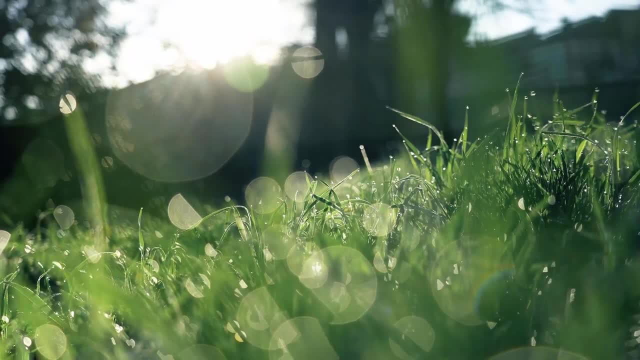 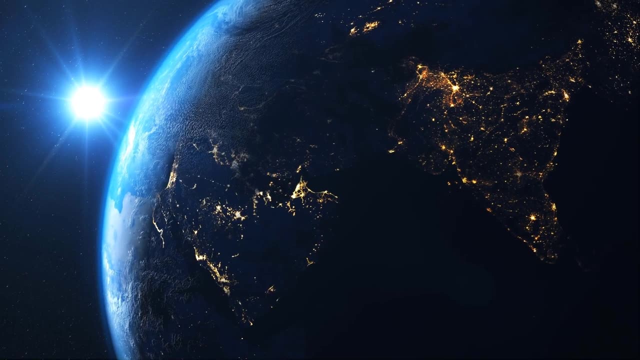 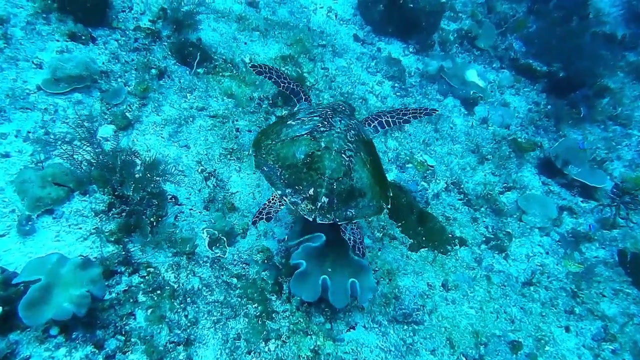 serving as the base of the ocean food chain and regulating the global climate. Without phytoplankton, life on Earth would be drastically different and possibly unsustainable. By protecting the ocean's health, we can help ensure the continued survival of these vital organisms and the ecosystems they support. So the next time you take a breath of fresh air, 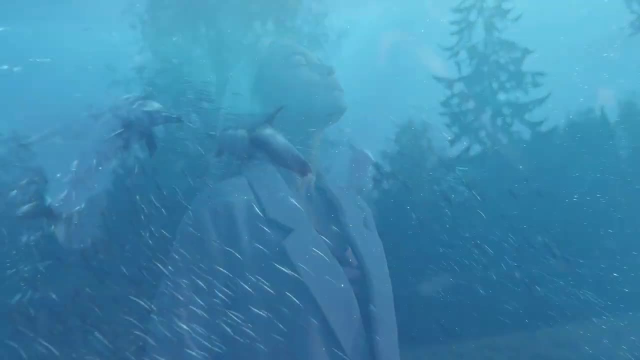 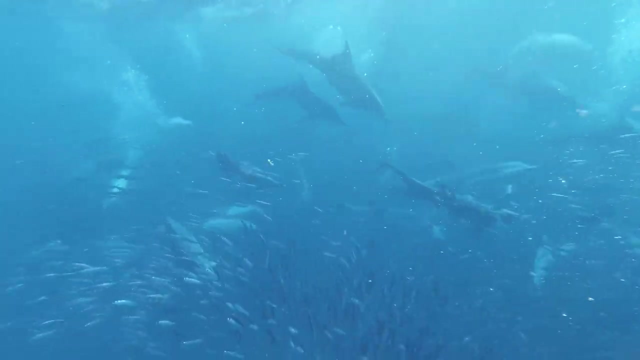 thank the phytoplankton for their hard work. If you enjoyed watching this video, don't forget to like and subscribe to our channel for more exciting ideas. Thanks for watching.